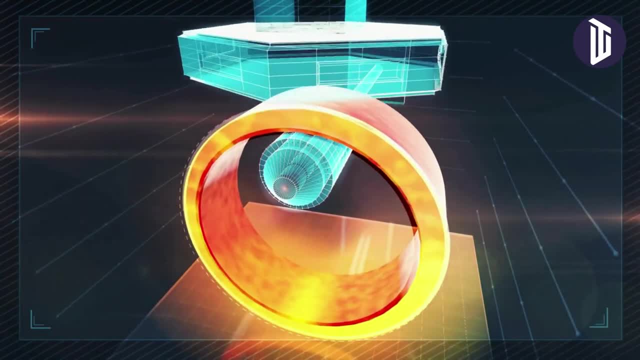 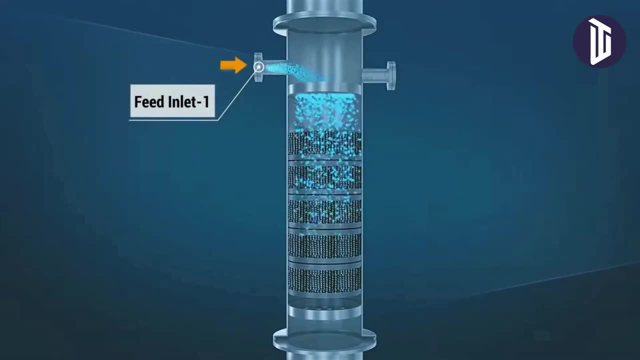 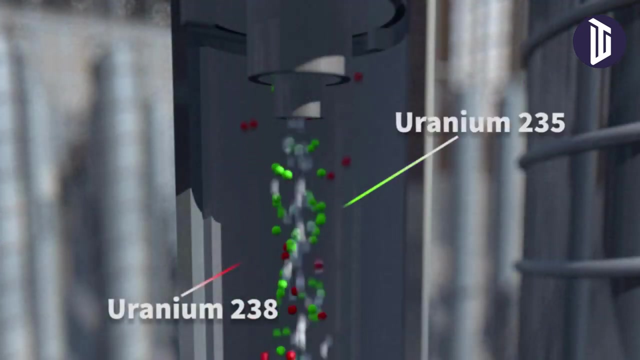 and the fabrication of thick pressure vessels presented formidable challenges. In contrast, the essential technology for pressurized heavy water reactors centered on heavy water production. The mastery of the intricate and energy-intensive process of uranium enrichment was perceived as more difficult and strategically sensitive. 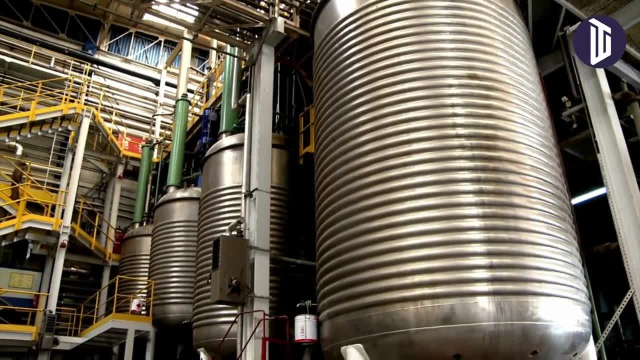 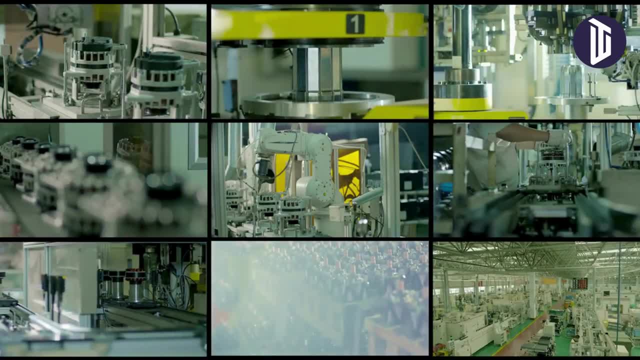 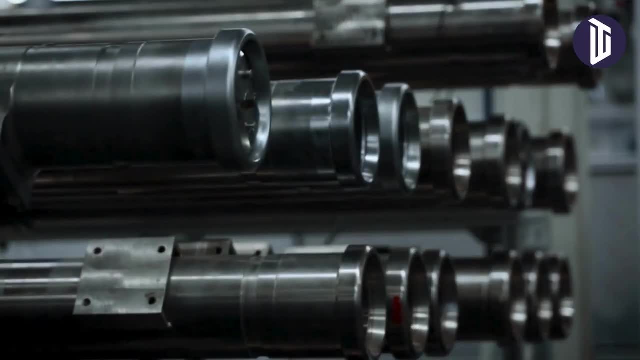 rendering it less accessible. On the flip side, the production of heavy water from natural water through a chemical exchange process appeared more feasible, aligning with the technological infrastructure available in the country at that time. PHWR's, being of pressure tube-type construction, did not require large and thick. 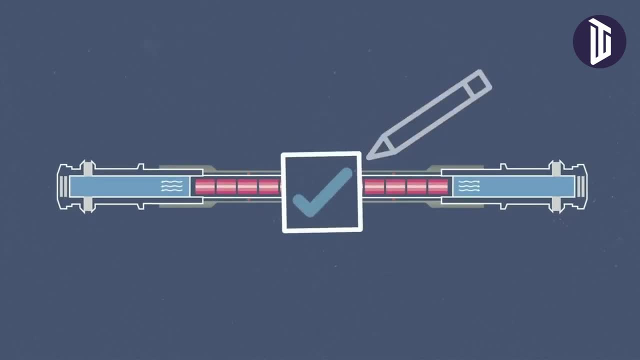 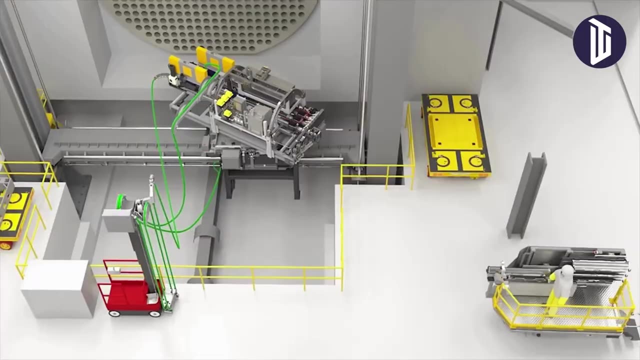 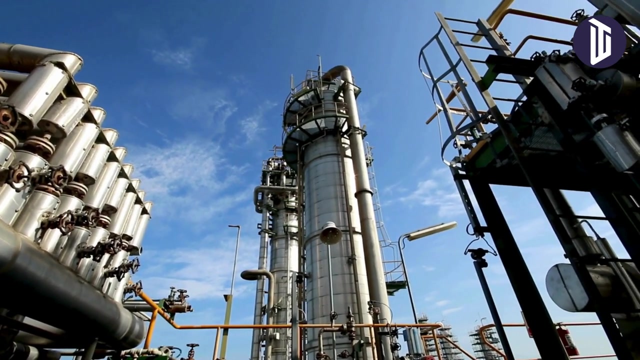 pressure vessels and therefore were not difficult to manufacture in the country. The familiarity of Indian scientists and engineers with research reactor Cyrus was also a factor in favor of the selection of PHWRs. Besides, a heavy water plant was also operational at Nangal in North India, producing about 10 tons of heavy water per year. 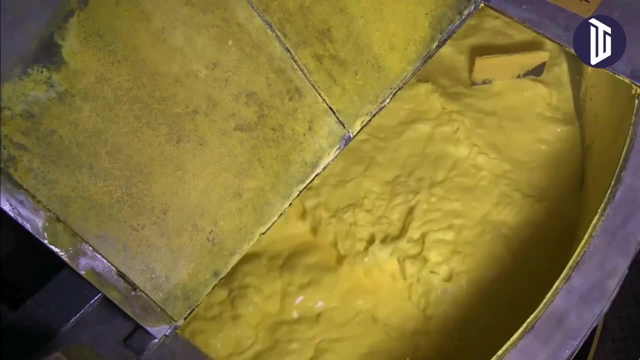 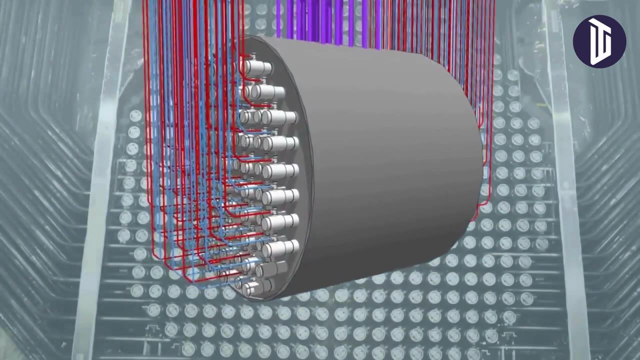 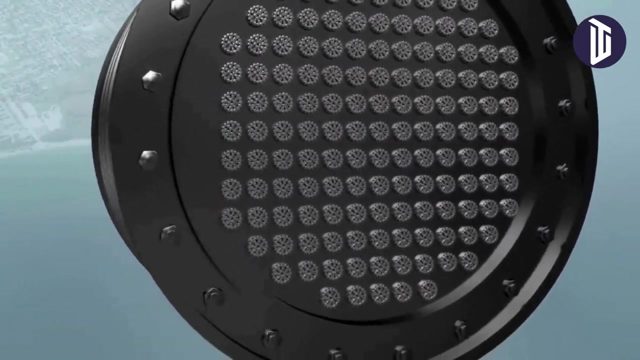 India's natural uranium reserves are limited. Hence it is essential to prioritize the efficient utilization of naturally occurring uranium in the first-stage reactor of the country's nuclear power program. The PHWR-type reactor holds key advantages over PWR and BWR counterparts. that favors India's nuclear program. To delve into these advantages: 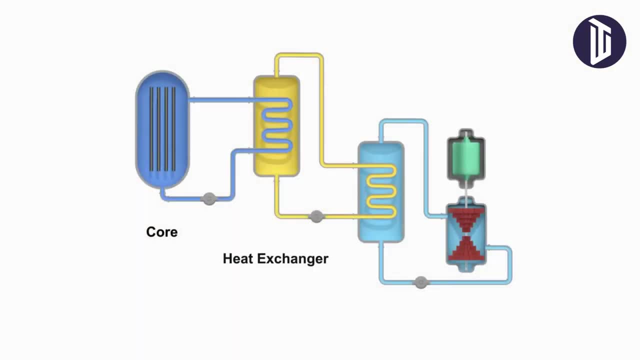 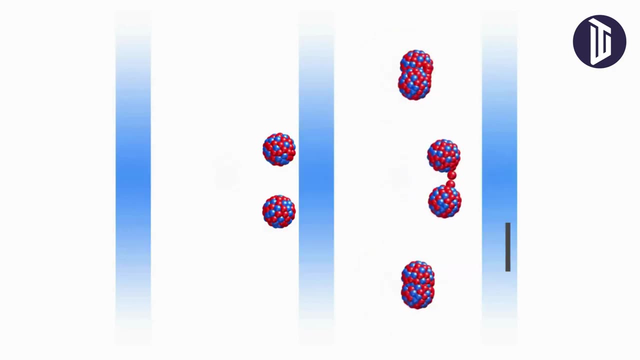 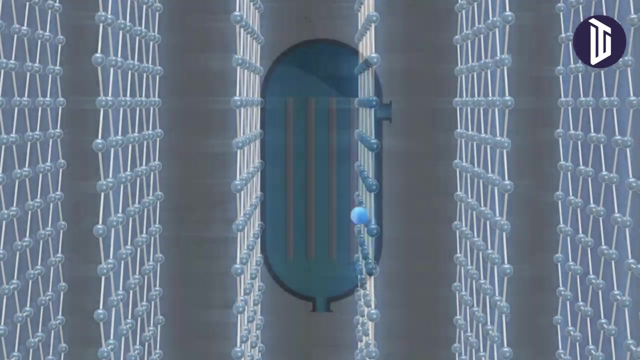 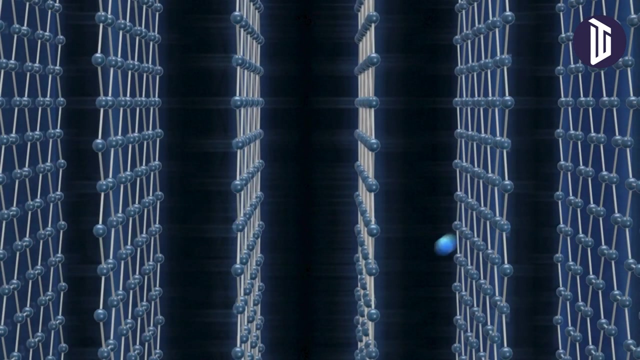 it's essential to familiarize ourselves with fundamental nuclear reactor terminology, including concepts like moderator, fissile material and fertile material. A moderator is a material placed in a nuclear reactor core to slow down neutrons produced from fission. Moderators are made of materials with light nuclei, like beryllium and graphite, that slow down neutrons through a. 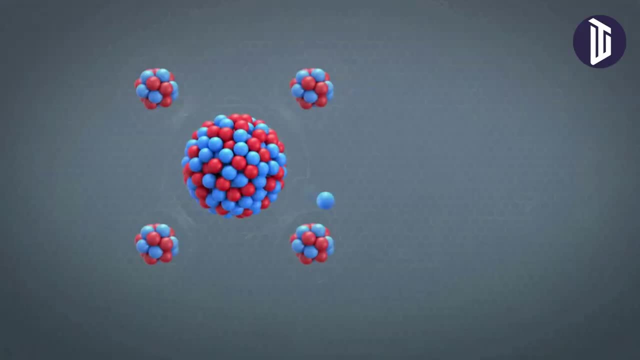 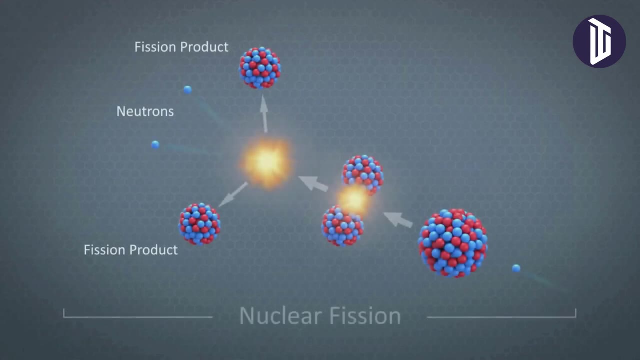 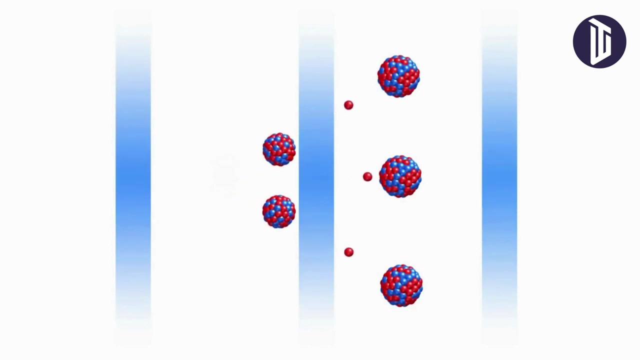 series of collisions. By slowing the neutrons down, the probability of a neutron interacting is greatly increased, thereby maintaining the chain reaction. Fissile material is material that can undergo nuclear fission when struck by a neutron of low energy. Fertile material is a material that, although not fissile itself, can be converted. 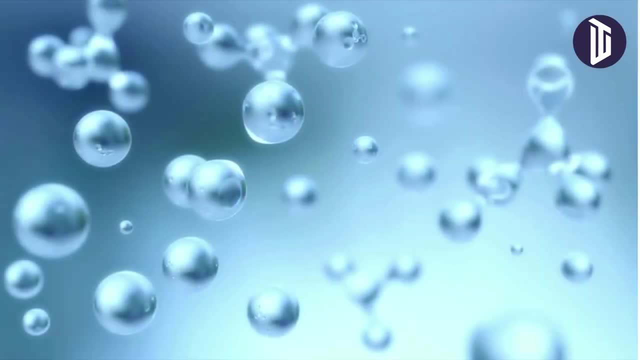 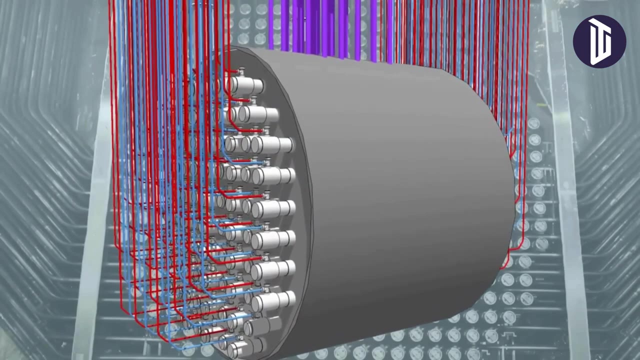 into a fissile material by neutron absorption. Heavy water is a type of water where the hydrogen atoms contain an extra neutron, making it denser than regular water. The pressurized heavy water reactors employ heavy water as a moderator, utilizing deuterium, an isotope of hydrogen. 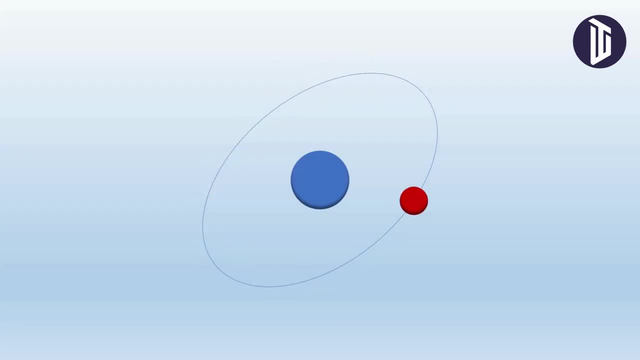 containing an extra-neutron instead of regular hydrogen found in normal water. Heavy water demonstrates superior efficiency in filtering the energy available in the nuclear reactor. Precisely nothing can remain vital to reduce environmentalapse or increase its upward growth rate, Which is a fundamental 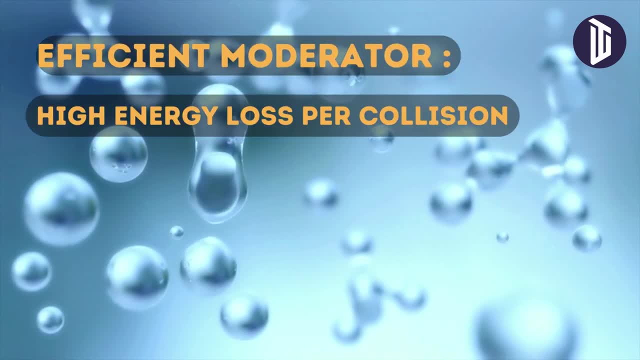 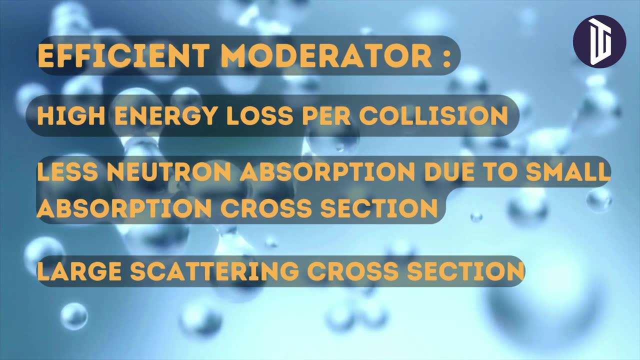 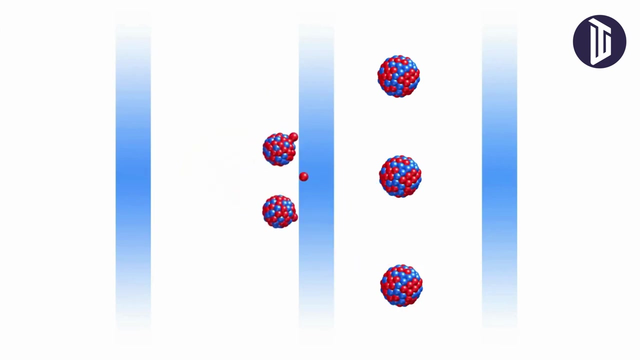 superior efficiency in reducing neutron energy and absorbing fewer neutrons compared to regular water. This feature establishes heavy water as an enhanced moderator in the reactor system, improving its capability to moderate neutrons more effectively. Consequently, this improved moderation increases the probability of initiating fission in uranium-235 without the need for fuel. 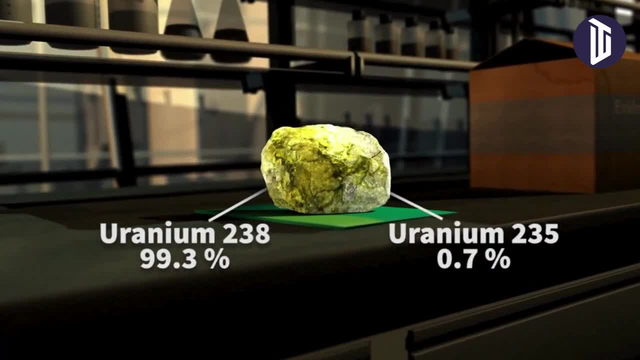 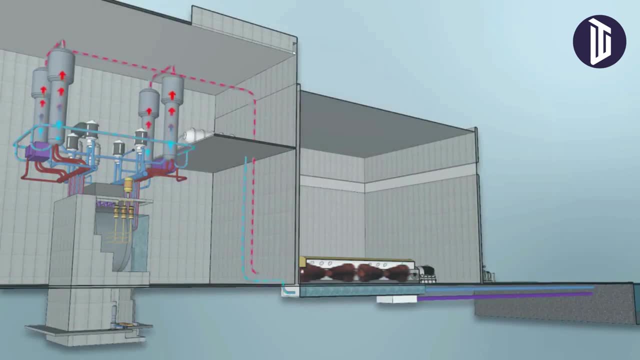 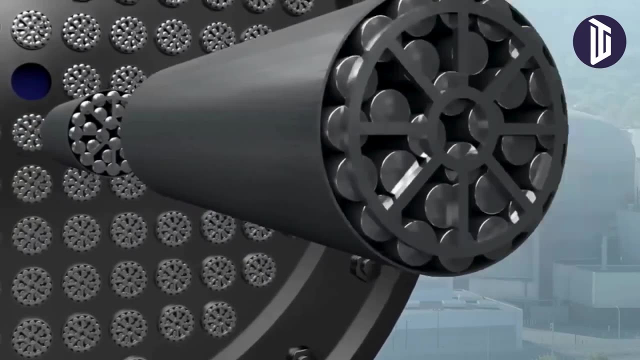 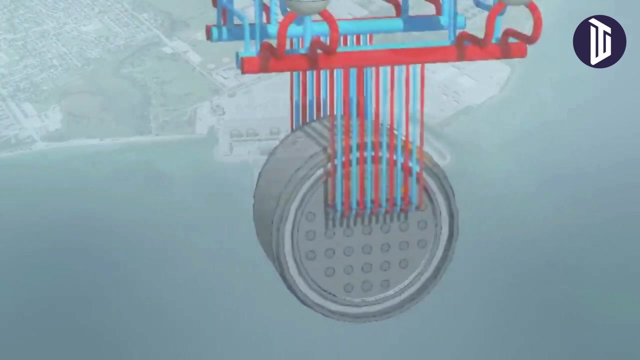 enrichment. Enrichment involves enhancing the concentration of fissile uranium within the fuel. This distinctive characteristic of PHWR-type reactors is advantageous for India's nuclear program, enabling the use of natural uranium instead of enriched uranium, as required by PWR and BWR reactors that use light water. Furthermore, PHWRs offer the capability of refueling while in 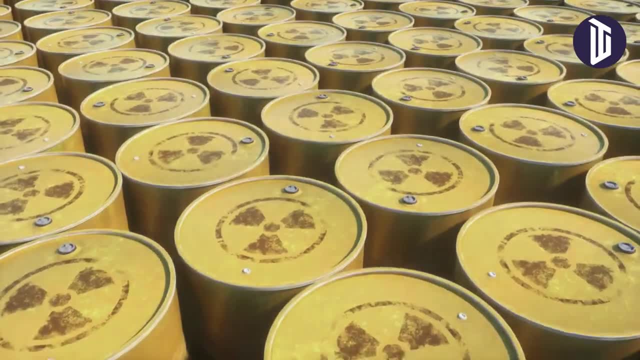 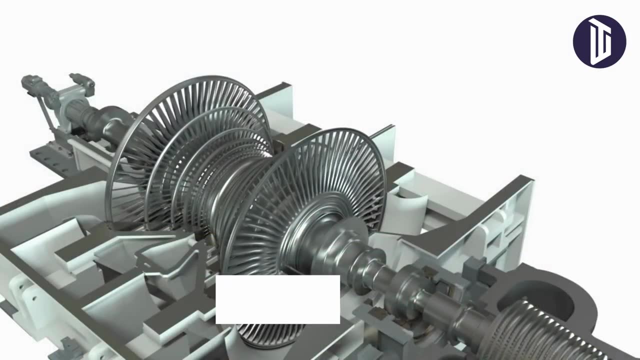 operation. maintaining high capacity factors. The domestic availability of natural uranium can sustain the pressurized heavy water reactor's power program, which can be used to produce up to a capacity of approximately 10,000 megawatts. Beyond this point, fueling additional 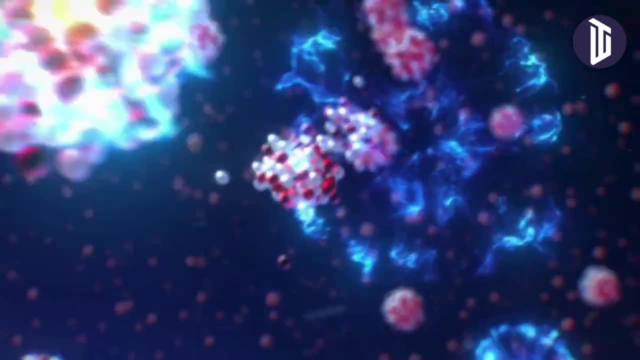 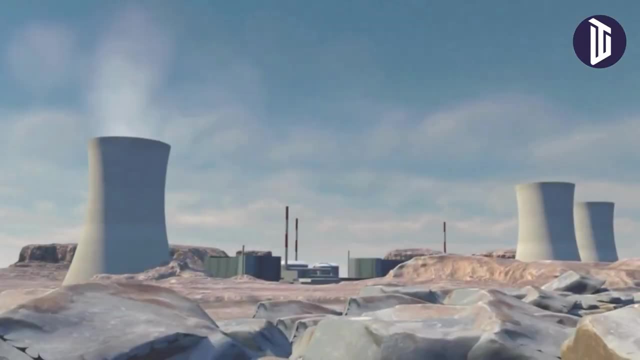 reactors becomes challenging and the program would be difficult to sustain. To address this issue, sodium-cooled fast reactors will be utilized in the second phase. The initial phase of India's nuclear power program revolves around the utilization of natural uranium in pressurized 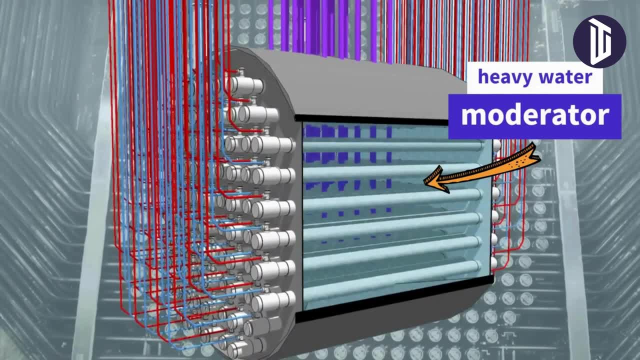 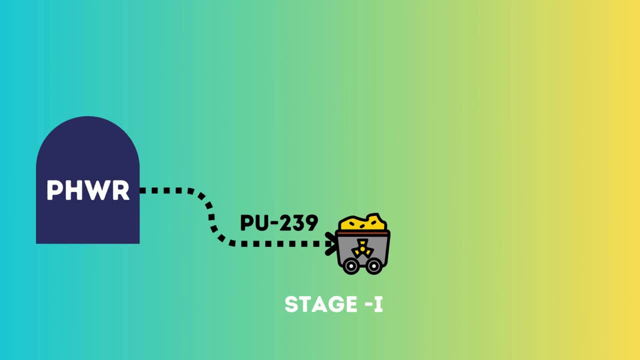 heavy water reactors. employing heavy water as a moderator, These reactors not only generate energy, but also produce fissile plutonium. In the second stage, plutonium-239 retrieved from reprocessed PHWR spent fuel combined with depleted uranium- mostly containing uranium-238, will be utilized in a 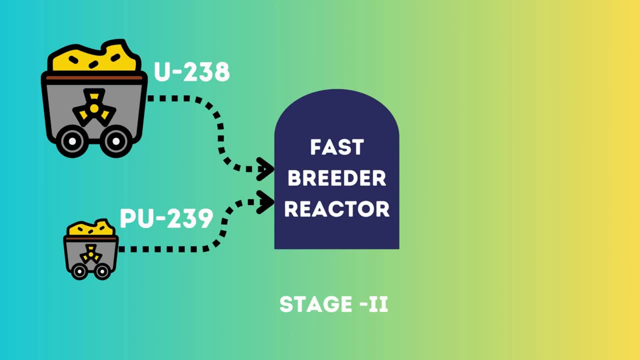 sodium-cooled fast reactor. These reactors, with their breeding capability, can generate more fissile material than they consume, ensuring a consistent supply of nuclear fuel for power generation. This is critical for sustaining a nuclear power generation, The second phase of India's 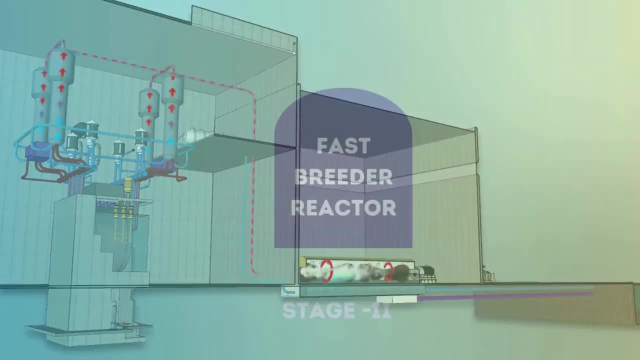 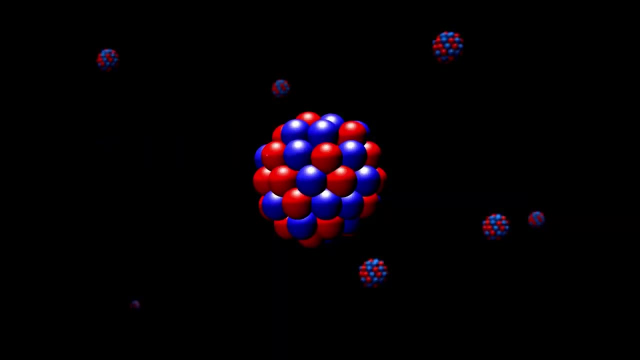 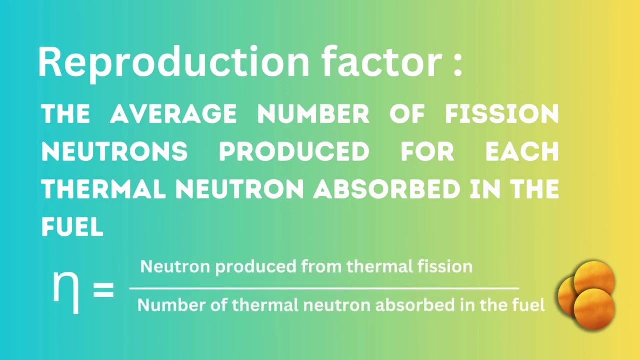 nuclear power program revolves around the utilization of natural uranium-238, or thorium-232,, depending on the number of neutrons generated in fission. This concept is expressed by the reproduction factor denoted by eta, representing the ratio of neutrons produced. 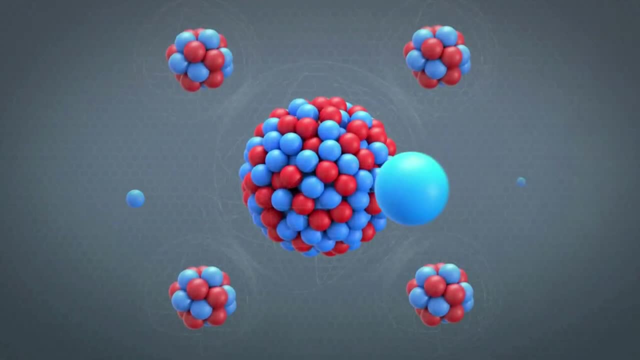 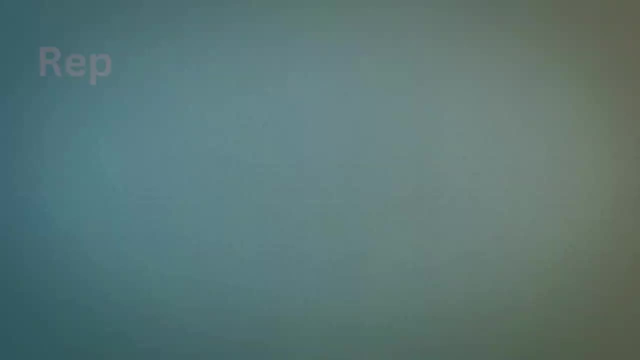 by the fission process to those absorbed. Besides one neutron, to continue the fission chain, additional neutrons would be used to convert the fertile nuclei to fissile nuclei. This factor must be greater than two, allowing for parasitic absorption of neutrons in other 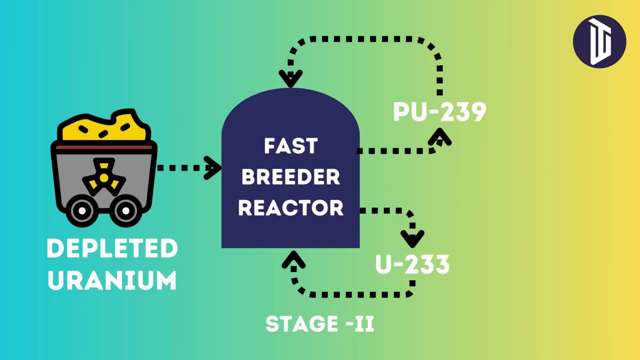 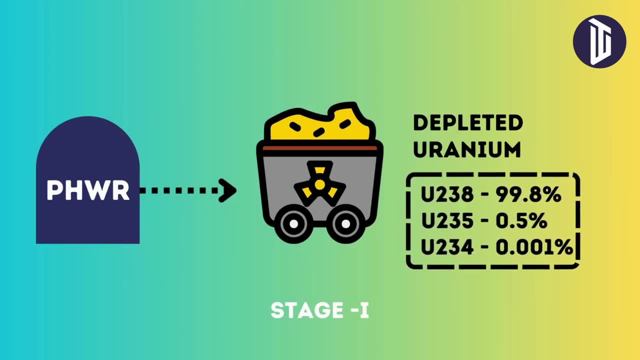 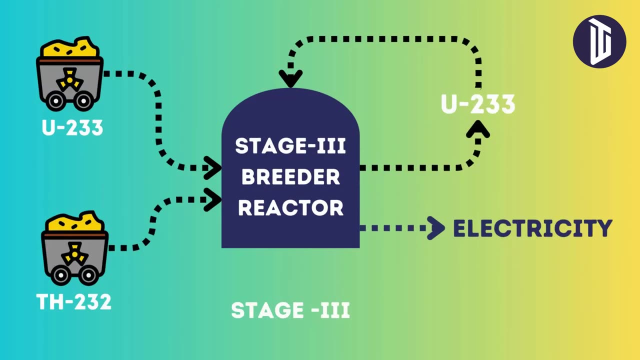 structural materials. It's important to note that India has the potential to generate up to 300 gigawatts of electricity using depleted uranium sourced from the spent fuel of pressurized heavy water reactors, which could sustain for approximately 100 years. The third stage is 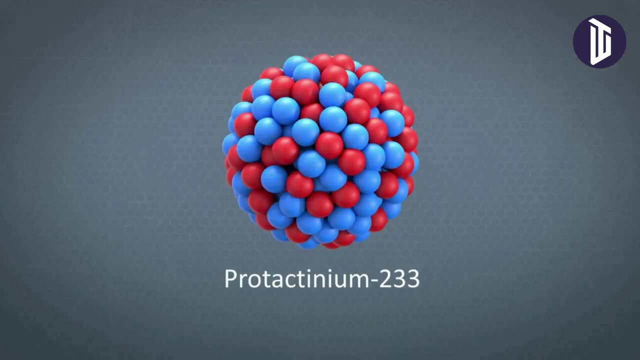 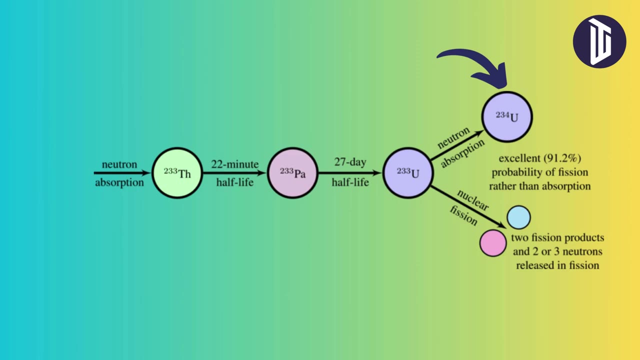 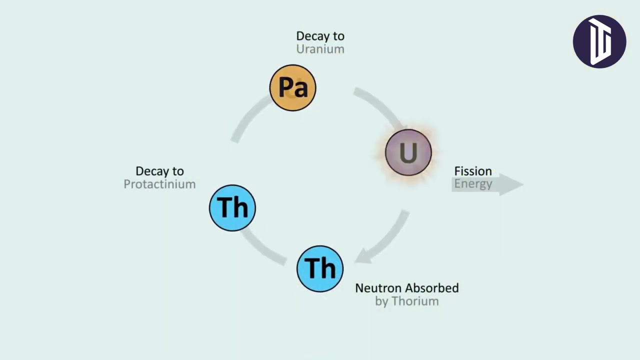 currently in the development phase, and challenges related to the presence of protactinium-233 leading to the formation of uranium-234 needs to be addressed. Additionally, the fissile material required for the third stage must originate from the second stage. The utilization of thorium is a 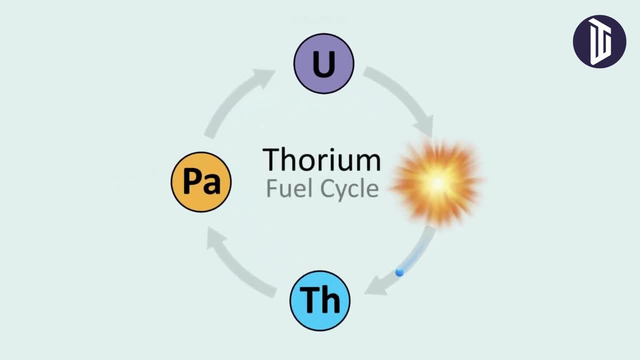 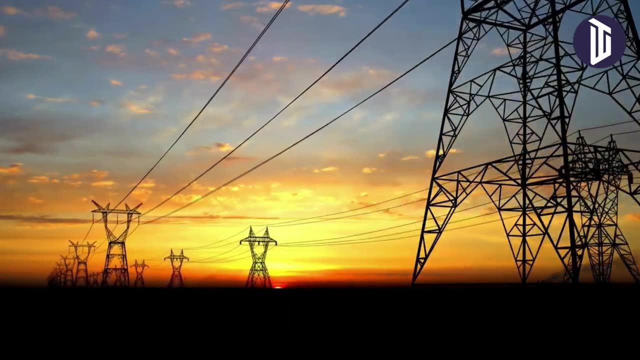 key consideration, given India's substantial reserves of this resource. India is also developing advanced nuclear technology to address its expanding power needs and ensure the security of its growing energy demand. India is actively engaged in the development of its nuclear power systems. India is working closely with the Department of Nuclear Engineering on development. 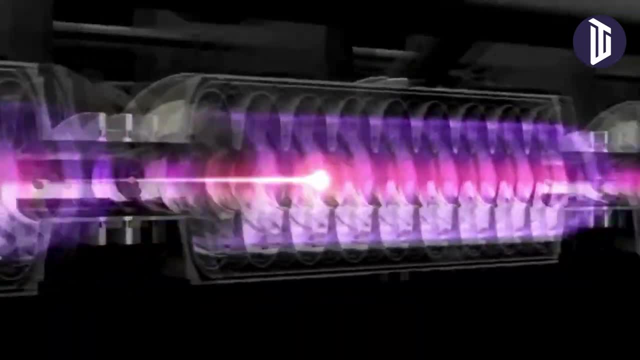 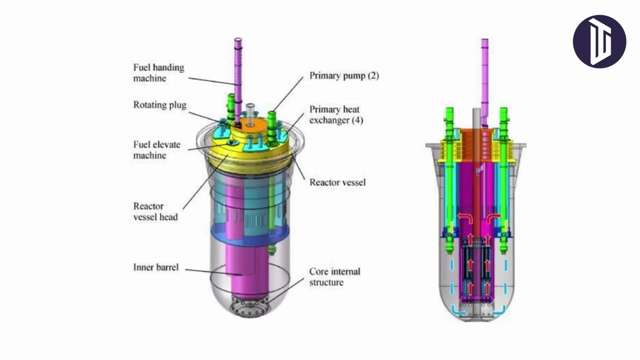 and development of accelerator-driven systems that will utilize natural uranium and thorium as fuel. The Department of Atomic Energy and Fermilab are collaborating on the design of these systems. The project will be the world's first ADS reactor and will produce green electricity from India's 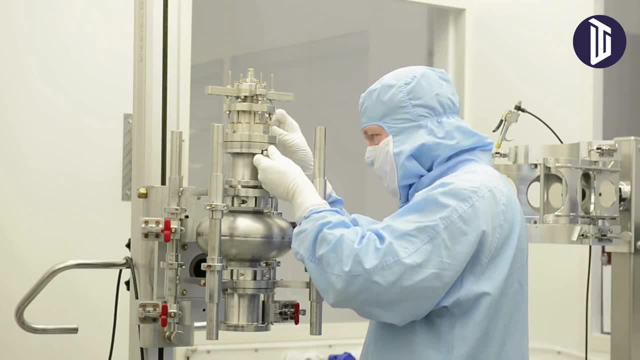 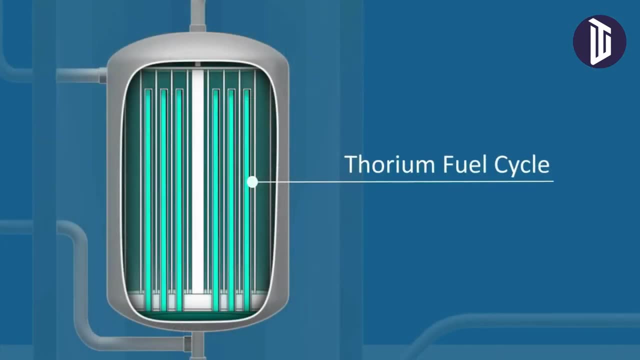 thorium reserves. Scientists from Fermilab and BABA Research Center will be part of the team. Furthermore, India's nuclear endeavors extend to diverse initiatives including the development of thorium-based reactors, advanced heavy water reactors and the development of new nuclear. 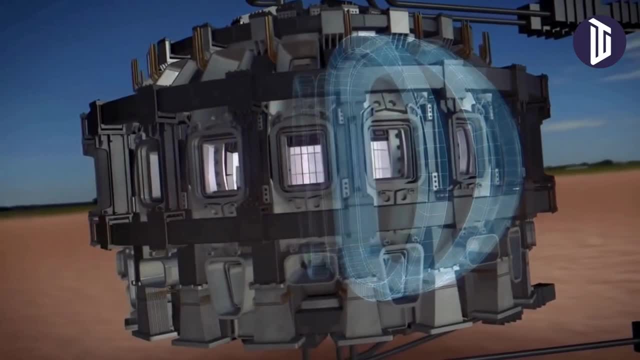 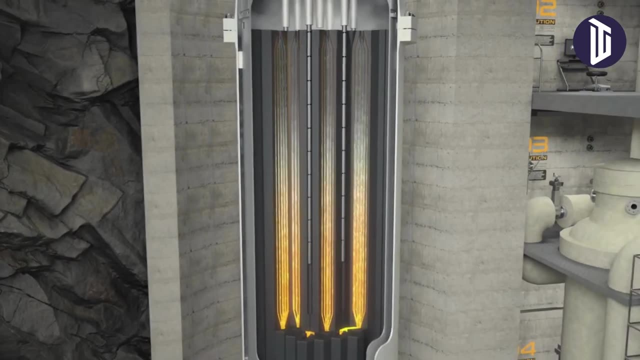 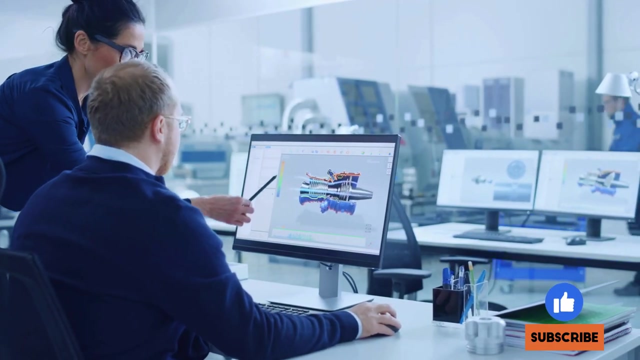 water reactors, fast breeder reactors, nuclear fusion research through the ITER project and the exploration of small modular reactors. These efforts collectively aim to ensure long-term energy security and optimize the efficient use of nuclear resources. Creating informative videos demands a tremendous amount of effort. Your support is crucial in fueling our motivation.